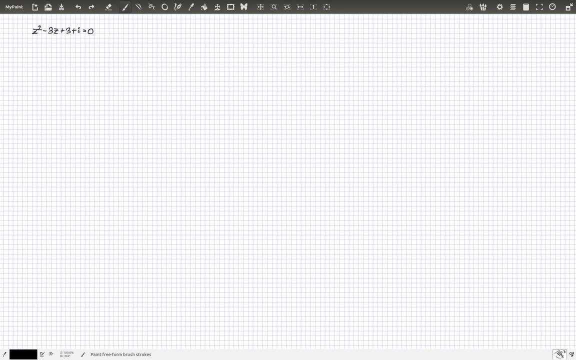 Hi, today I want to show you how to solve quadratic equation with complex coefficient. So our equation is written here. Our coefficient are: a is equal to 1, b is equal to minus 3 and c- it's complex- and is 3 plus i, where, of course, 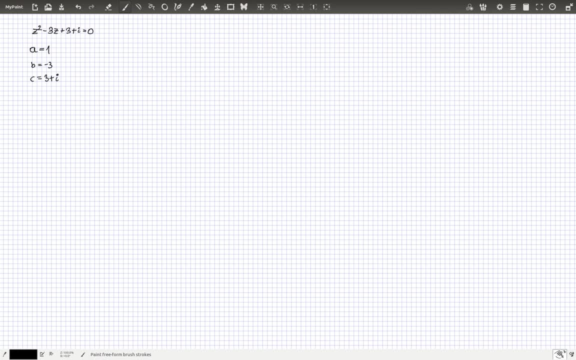 i is the square root of minus 1.. Okay, how to begin the solution? First of all, like in real case, we have to calculate Delta. Delta is b squared minus minus 4 times a times c. So if we use these values, it, 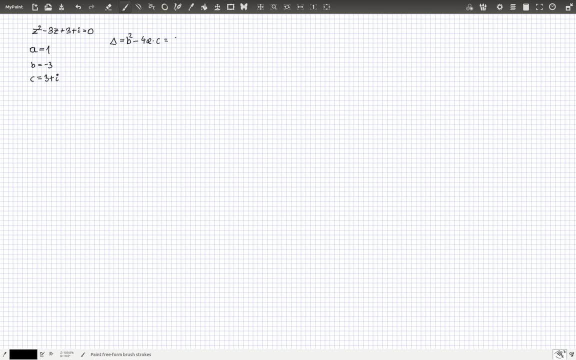 will be minus 3 to squared. squared minus 3 is 9, minus 4 times 1 and times 3 plus 1.. Okay, if we evaluate this, the answer will be minus 3 minus 4i. Okay, so our 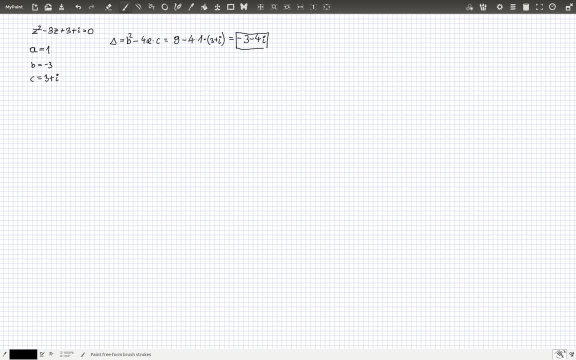 Delta is complex number. What we can do about it? Remember that in the solution for two solutions of the quadratic equation we have the following formula: minus b plus minus square root of Delta and divided by 2a. So to obtain the solution we have to know the square roots of Delta. 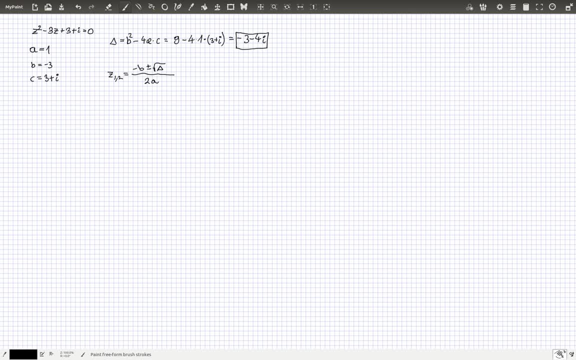 So how to obtain the answer: the square roots from Delta. Let's calculate it. First of all, let's assume that square root of Delta is some complex number. It's x plus ai, y, And, of course, x and y are purely real numbers. 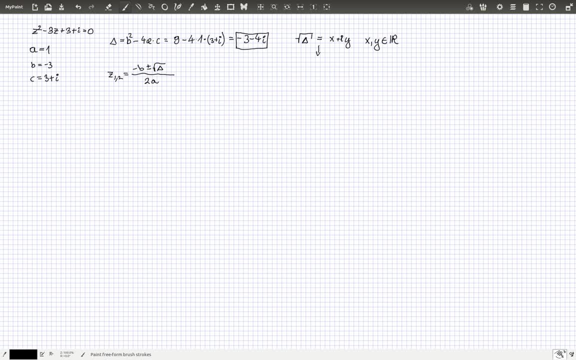 So the trick is to square the both sides of this equation, And what we'll get here? On the left side we will get Delta, And on the right side we will get x plus ai y squared. So if we calculate this using formulas for squared sum, we will get x squared plus 2x. 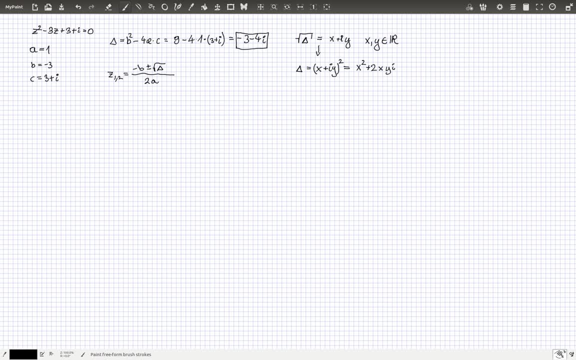 plus times y, times i and minus y, squared Because i squared, is minus 1.. So this is how this minus appears here, And let's rearrange the terms. Okay, So we know that our Delta is this number And we know that, and we will want to know the square root of Delta. 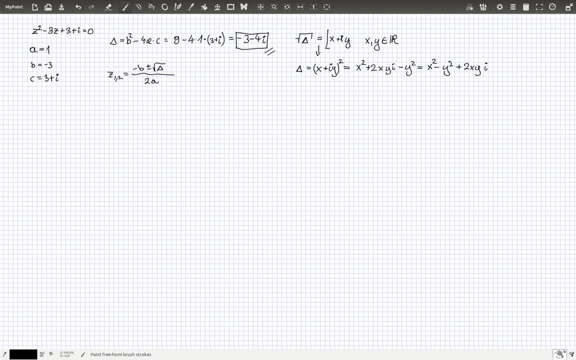 So the square root of Delta is x plus ai y, And we know that Delta is, We know that Delta is such a formula. So we can compare this to these two numbers, Because they should will be equal. Delta should be equal to this Delta. 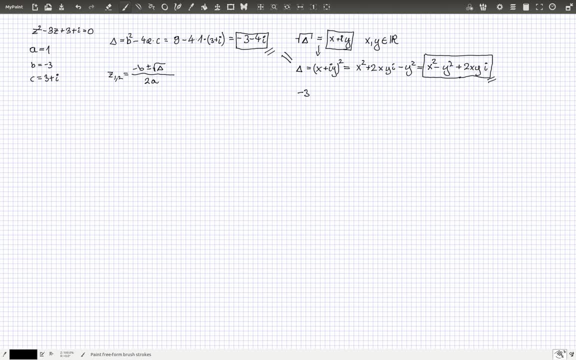 Okay, So minus 3, minus 4a, Delta should be equal to x squared minus y squared plus 2x times y- i. So this is true only if real parts of left hand side and right hand side are equal And complex parts of left hand side and right hand side are equal. 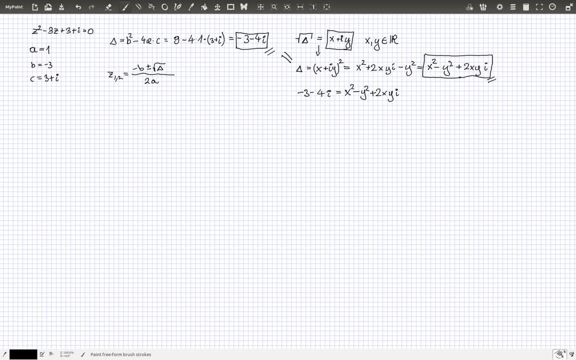 So This one equation will produce for us two equations. First is minus 3 from the left hand side should be equal to x squared minus y squared, And second, is minus 4 should be equal to 2xy. Okay, This is our set of equations. 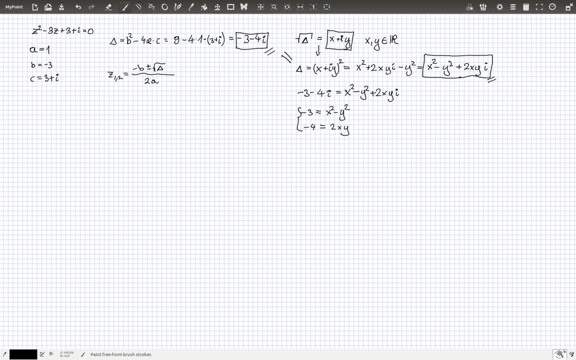 Now how to solve this. There is a mathematical trick To First of all Multiplies first equation by, By, for example, y squared And squared Both sides of sides of the Second equation. What we will get then? First, 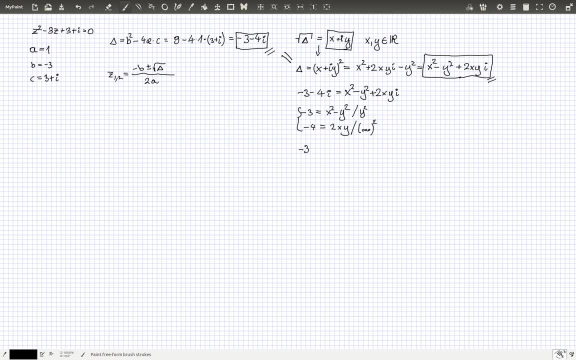 We will multiply by y squared. So on the left hand side we will get minus 3y squared, And on the right hand side we will get X squared, Y squared Minus y to the fourth. So This is our first equation. 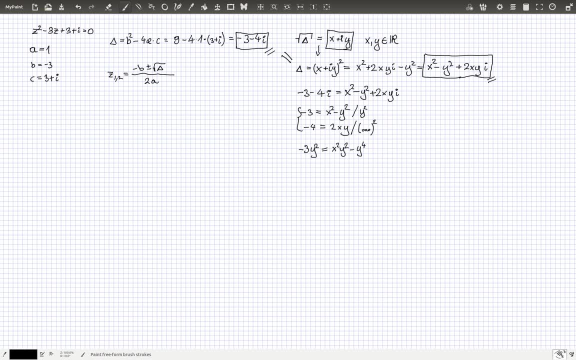 And second equation Will be squared. So on the left hand side we will get 16.. On the right hand side We will get 4.. 4x squared, y squared. Of course we can Divided both sides by 4.. 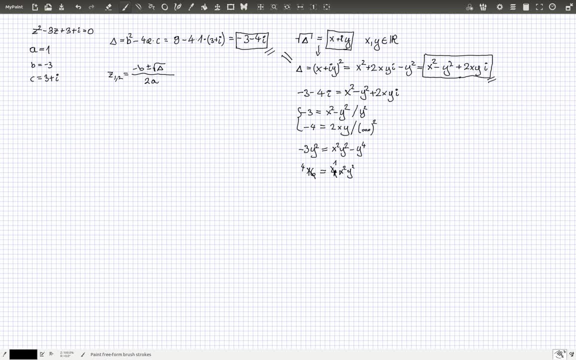 And we will get here 4.. And Here 1.. Okay, Why we would Like to do that, This Transformation, This multiplication and This powering of the second equation. Look, This term Is the same as this term. 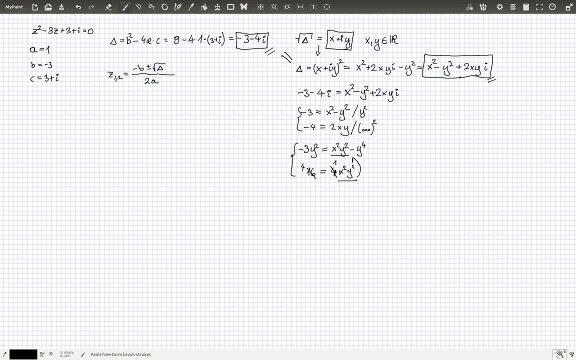 So we can plug Second equation Into first equation. So what we will get then, After plugging this We will get: Minus Y squared Is equal. We know that X squared times y squared is 4.. So we 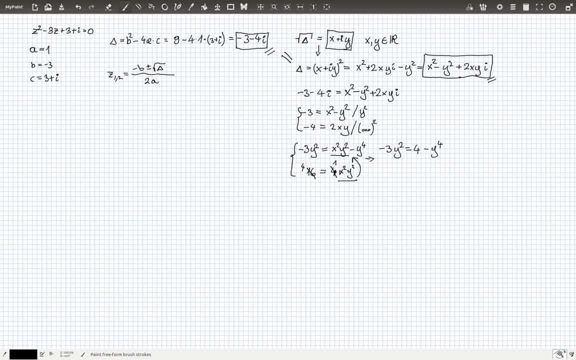 Write here: 4. Minus: y To the fourth power. Okay, Let's rearrange the terms. Let's move Right hand side to the left hand side, And then we will get Y To the fourth, Minus 3.. 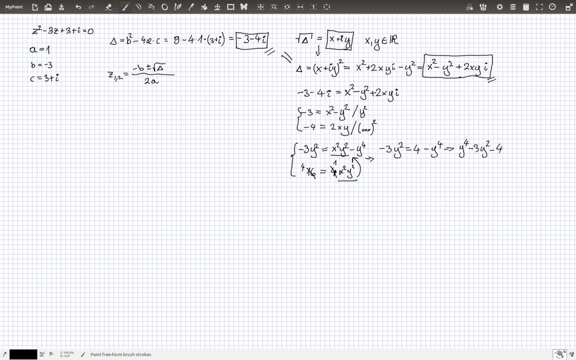 Y squared Minus 4. Is equal to 0.. So We get New equation And we have to solve it. To solve this set of equation For y and x, How to do that? We have to Make. 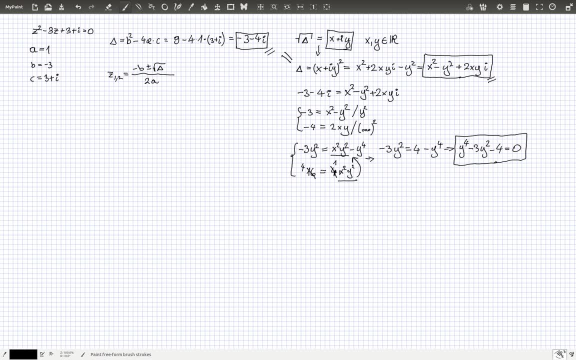 New Substitution. Let's call Y squared. Let's Call Y squared t. If we do that, The equation Will became T squared Minus 3.. T Minus 4.. Okay, We know how. 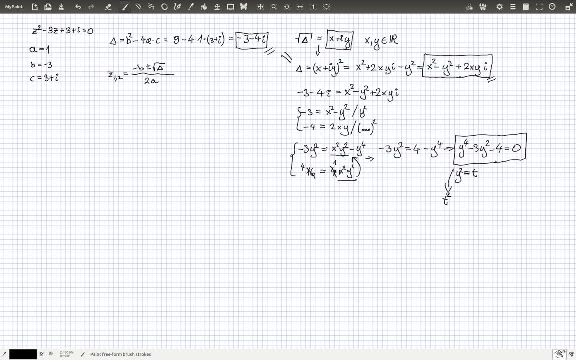 To solve This set of equations. So We have to Make New Substitution. Let's call Y squared. Let's Solve This set of equations. Okay, We know how To solve This equation. Let's do that. 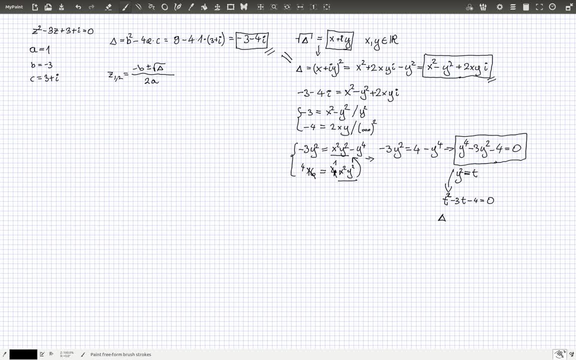 Let's calculate Delta. But this is Not the same Delta As before This. Let's Call it Delta Prime. It's 9. Minus 4. Times 1. Times 4.. 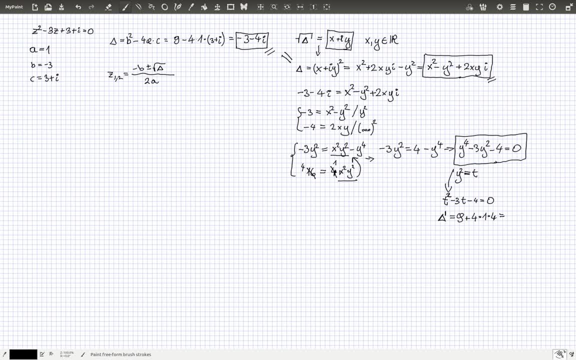 Minus 4.. So This Is 25.. So We can Calculate T1.. T2.. It's Minus B, So It's 3. Plus Minus Square. 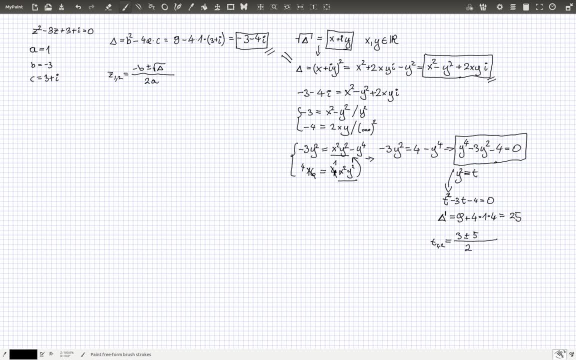 Root From 25. It's 5. Divided By 2. A, A Is 1., So It's 4.. And The Second Solution, T2. Is 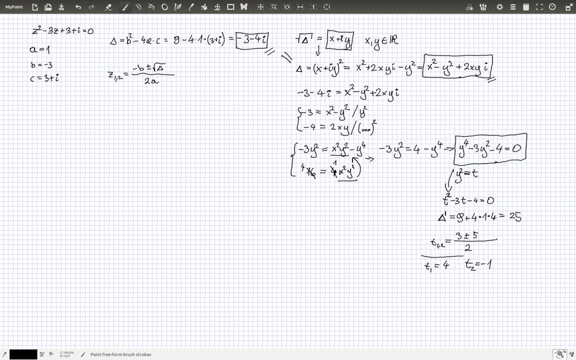 Minus 2.. Divided By 2. It's Minus 1.. Okay, So We Found Solution For The T And We Was Looking For The. 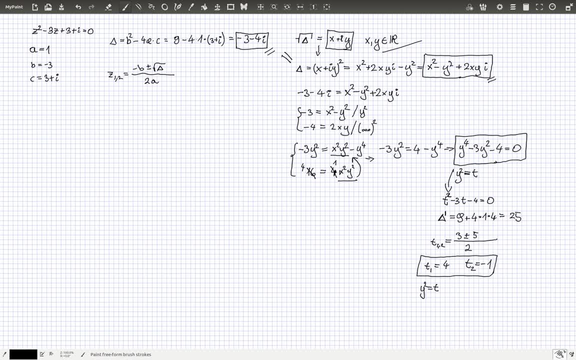 Y Here We Assume That Y Is Real Number, So Can Y Squared Before? Yes, Can It Can Before. So Y Then Is Equal To. 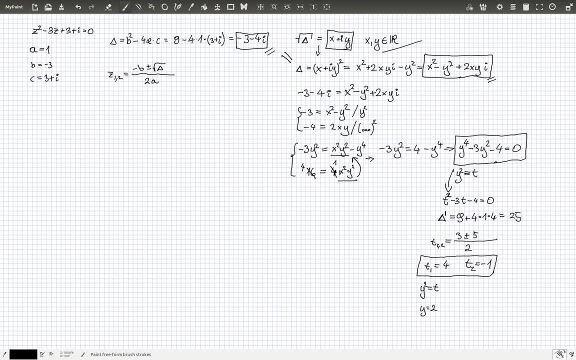 And Can Y Plus Minus I. But As We Said Before, As We Assume, Y Is Real Number, So Only Solution Is Y Equal To 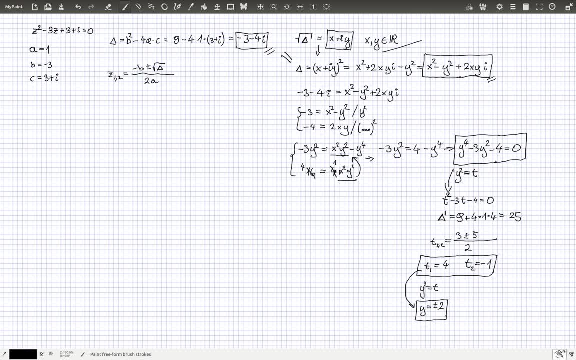 Actually Y Equal Plus Minus 2.. Okay, This Solution Of This Equation Is Plus Minus, Plus Minus 2.. And From From This Equation, 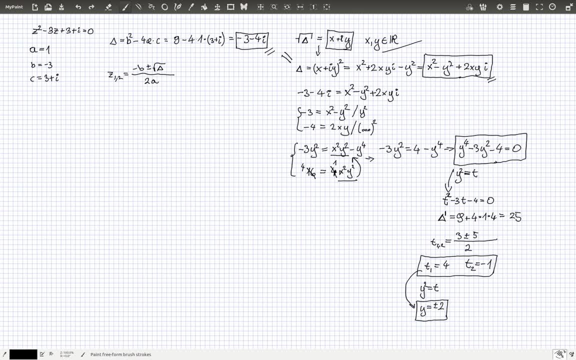 Actually Not From This, From This Equation. Let's Divide It Before Using It By 2. Y, So We Know That X Is Minus 2.. 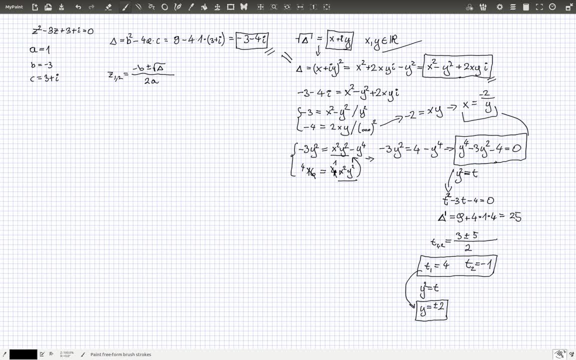 Divided By Y. Okay, Let's Use This Here. Oh Sorry, Let's Use It Here, And What We Will Get? We Get This From This. 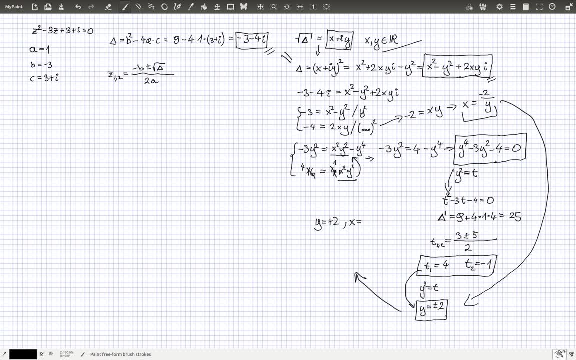 Equation From This: X Is Equal Minus 2.. Divided By Plus, 2. Is Minus 1. And For For Y Equal To Minus. 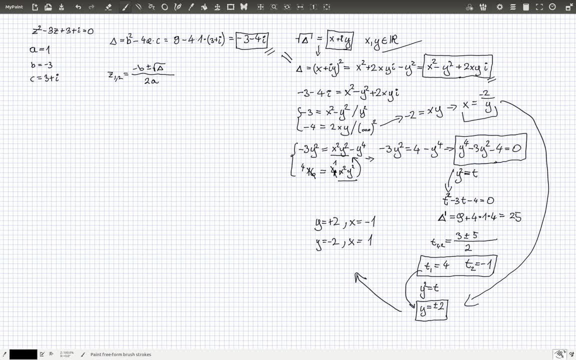 2. X Is Divided By Uh. Looking For The Solution Of This Set Of Equation? Uh Okay, So Let's Get Back To Uh This: 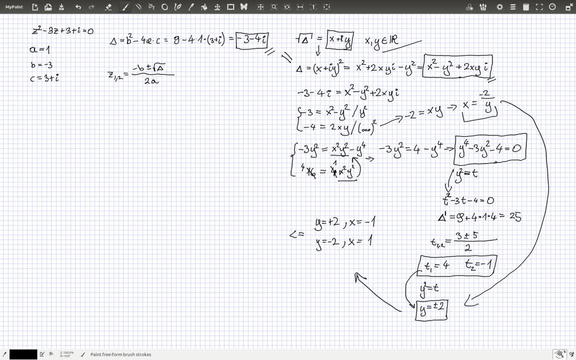 Formula. Uh. And One Thing To Notice: Uh, We Solve This Equation That Is: Um Is Minus 1., Plus 2. I And The Second. 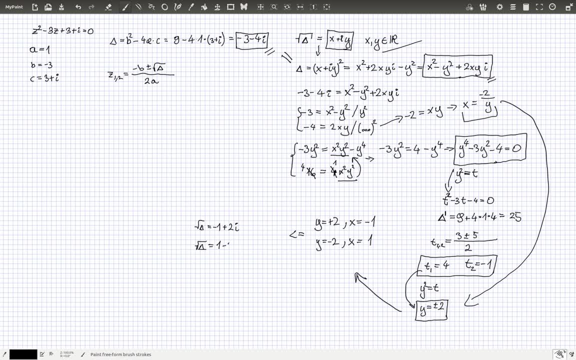 Solution Is Um One Minus 2. I Um, Of Course, Uh, We Know That From Delta. But Uh, Here We Have Plus Minus, Uh, 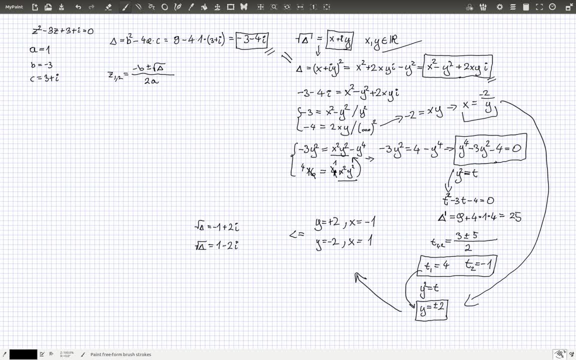 Plus Minus Square To Delta. So, Uh, The Argument Is That We Don't Have To Um Use Here Plus Minus, Uh, The Main Theorem. 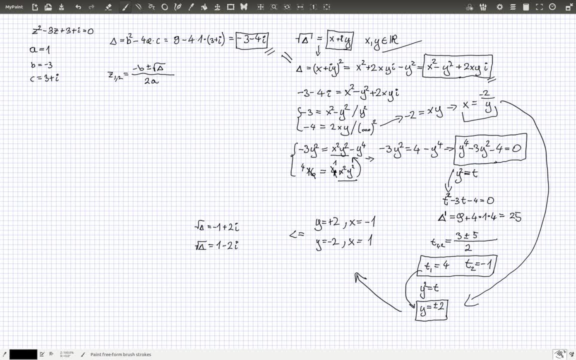 In Algebra It States That The Um, This Equation Of The Second Degree, Equation Polynomial, Uh, Have Only Two Solutions. So Uh, This Solution If Equation: 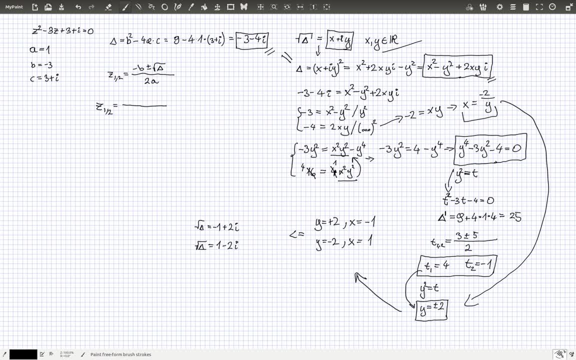 Will Be Um Minus Three, Minus B It's Plus Uh, Three Plus Minus. First, Square Root Of Delta, Divided By Two, Oh Actually. 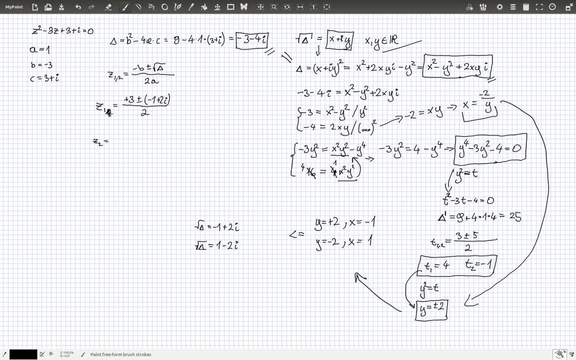 I Want To Write Here One- Oh Sorry, It Should Be Plus Here- Um Plus One Minus Two, I Divided By Two. So If We 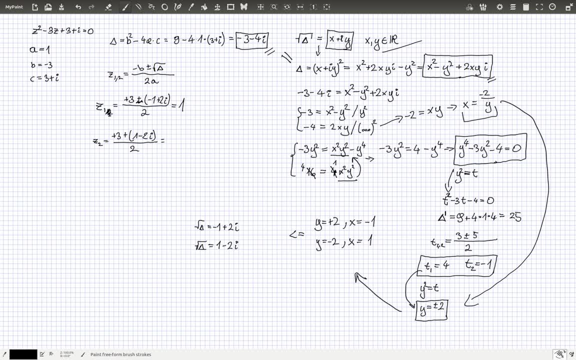 Evaluate First And Second, We Will Get Uh Three Minus One, And Second Is Four. Divided By Two Is Two Minus Two, I Minus. 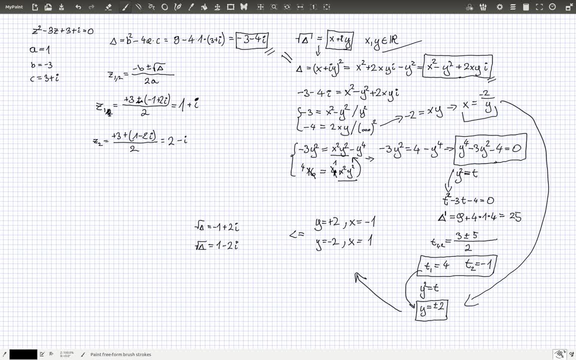 Two I Divided By Two Is Two Is Just I. Okay, So One More Thing We Can. We Can Rewrite This As Follows: Z Minus. 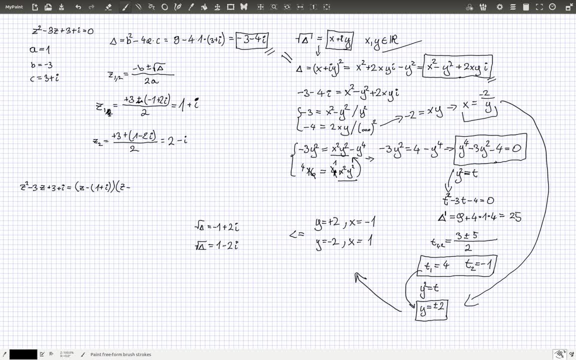 One Plus I And Z Minus Two Minus I. And If We Will Multiply This Uh Formula Here, We Should Get Answer Your Problem With. 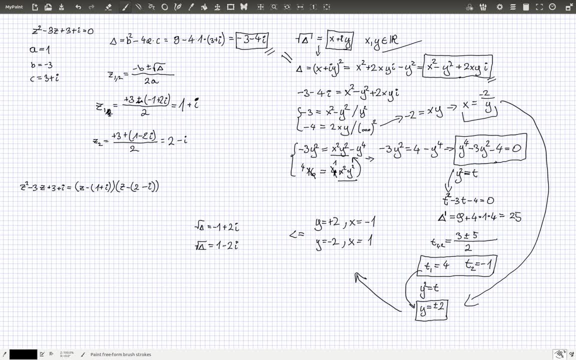 Algebra For Solving The Polynomials Of The Second Degree. Thank You, Take Care.